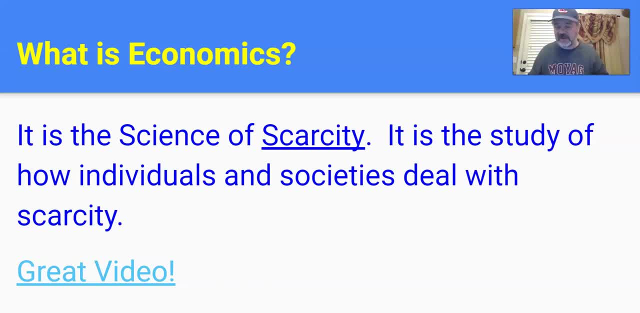 societies deal with scarcity. There, you know, there's not a lot of stuff out there, There's not an unlimited amount of anything, not even air, And so economics is the study of human behavior as we look at this idea of scarcity. There's a link on here which I'm going to link on this. 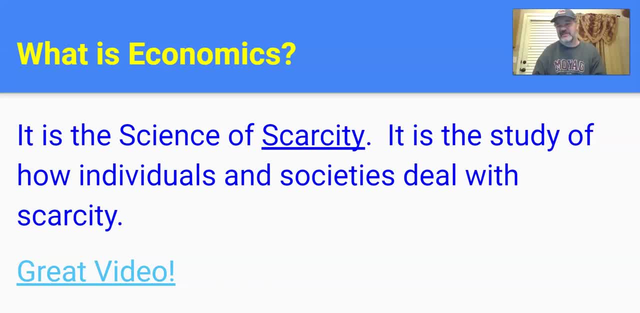 YouTube video. I highly recommend you watch it. It's a little corny but it's from Crash Course and it's a really good little introduction to what economics is, And so this will be the first video link that I'll put on this YouTube explanation of unit one. We're going to be 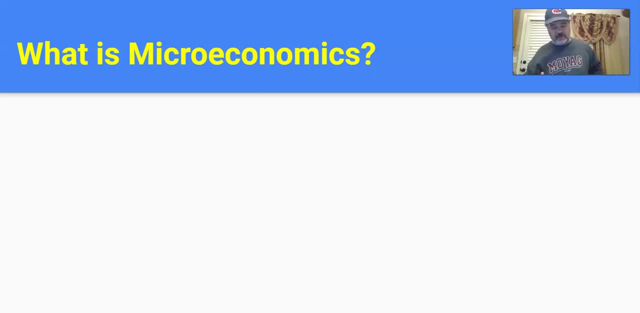 looking at microeconomics And macroeconomics. And let me start with what microeconomics is, And it's pretty simple. It's the study of small economic units such as individuals, firms and industries. We're going to take a look at things very, very small in our economy as we look at microeconomics Now. 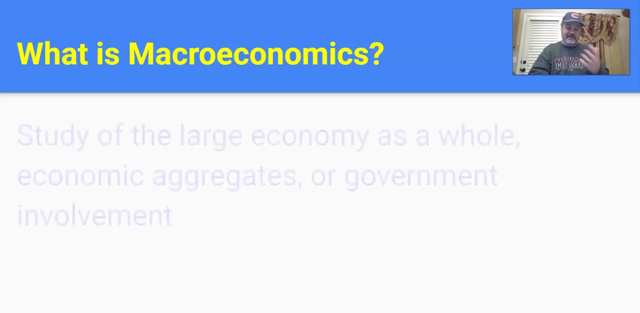 you can kind of figure that you already know what macroeconomics is going to be. That's pretty easy. It's the study of the large economy as a whole, economic aggregates or government involvement. Now I think it's kind of important to know what an aggregate is. An aggregate is when you take 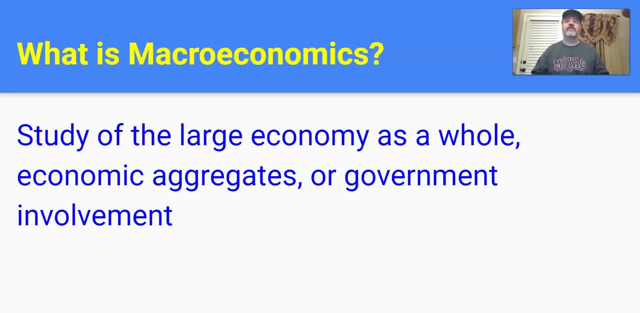 the collection of all those little things, all the people, all of the industries, all of the businesses, And if you put them together and you're looking at the economy as a whole, that becomes the aggregate. Okay, And of course you got to throw in government, because government has. 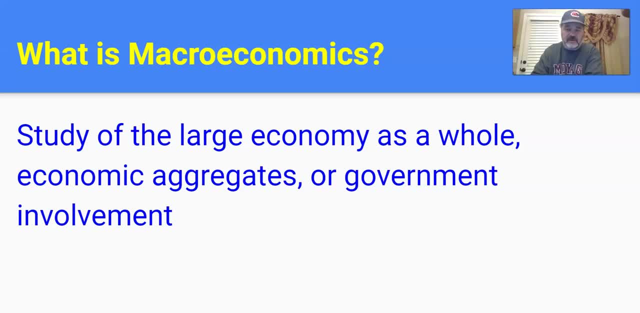 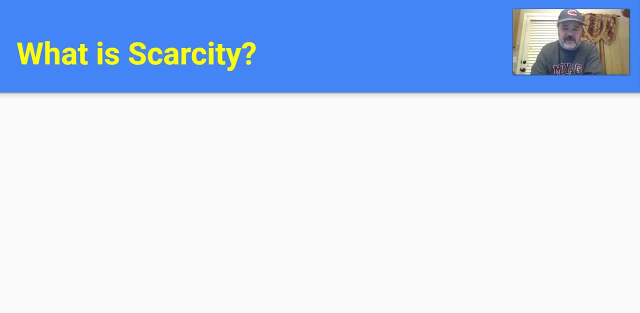 a lot of effect On the economy, even in- I mean in every country, And so we're going to take a look at that as well. So what exactly is scarcity? I mean, you know what it is, but what is it in terms of economic? 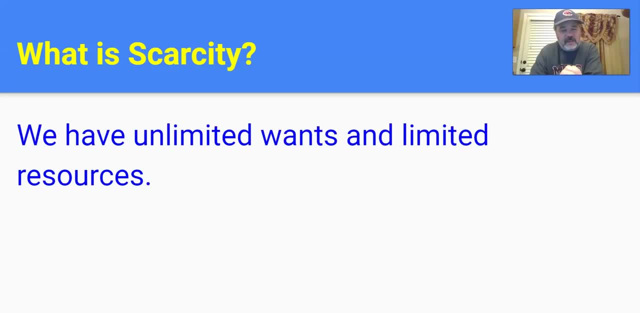 how it deals with economics. Just remember this: we have unlimited wants and we have limited resources. I mean it's kind of interesting. I mean, if you think about it, you know you're going to be a poor college student. You're going to be eating ramen noodles. You're not going. 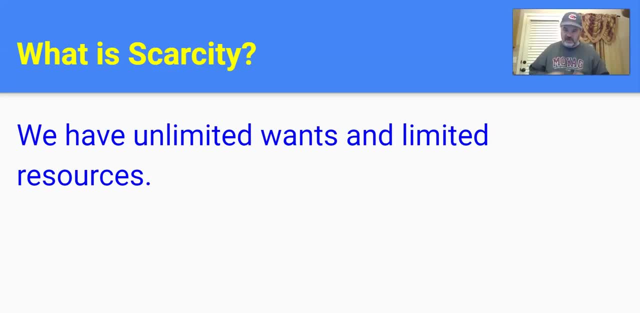 to have a lot of money on you And yet you're going to survive, You're going to make it, You're going to, you're going to, you know, get through to get your degree and whatnot. Well, when you get, 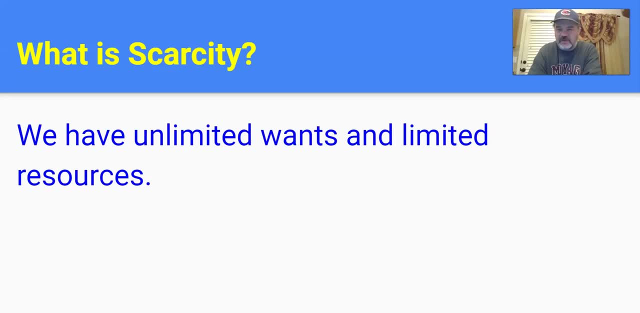 out of college and let's say, you get a real job- job okay- And you're making, let's say, $40,000 a year. You're going to make $40,000 a year. You're going to make $40,000 a year. You're going to make. 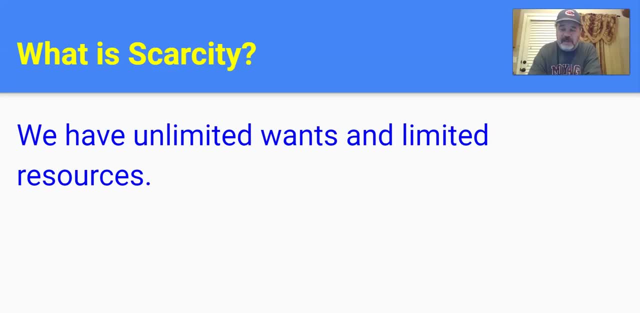 starting getting out of college, which is not a lot of money, but I mean it's a good starting salary. Are you going to start spending more money or are you going to stay the same as you were in college And and then actually you're going to be spending a lot more money because you have 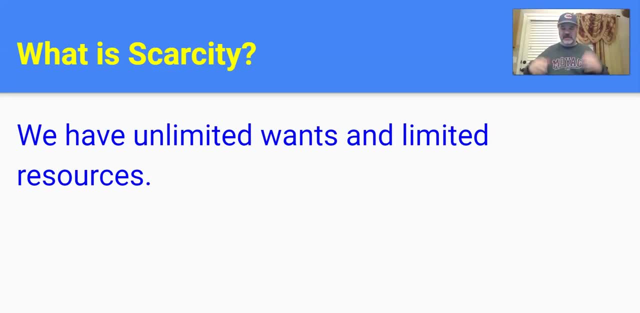 unlimited wants. Then suddenly you land that big, big job And all of a sudden, man, you have proven yourself and you go from 40,000 to $250,000 a year. Well, when you do that, what are you going to do? 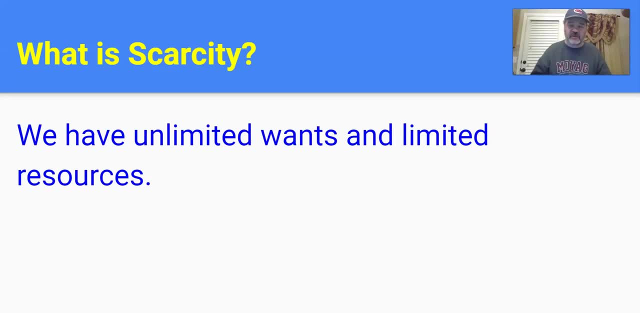 Are you going to still live the lifestyle of the $40,000 a year person or are you going to start spending more money? And the answer is: you're going to start spending more money because you have unlimited wants. And the problem out there is: there are limited resources And we're going to be. 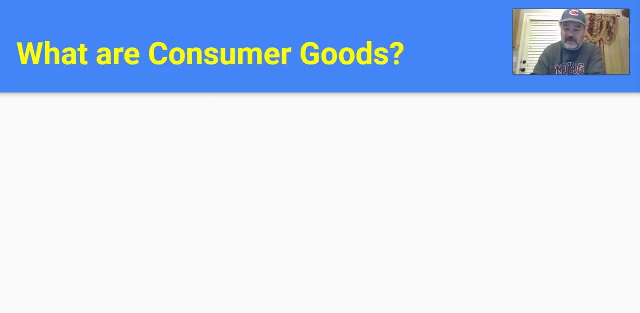 talking about that through the course of this semester. Now, when we look at those resources and things, we're going to look at something called consumer goods, and you're going to need to know what this is. Consumer goods are goods that are created for direct consumption. Okay, 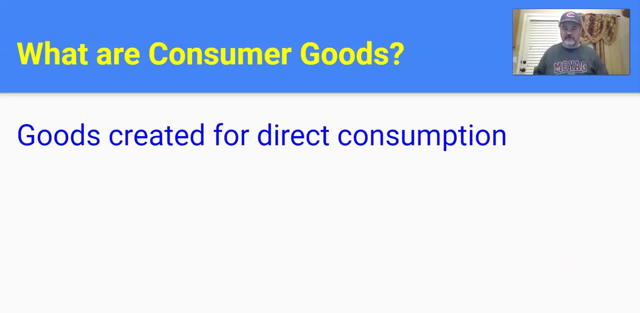 For example, and let me get you a good example like this: Uh these, when you get old, like me, uh, you need some reading glasses from time to time. Uh, this is a consumer good. Okay, This is for my direct consumption right here. Uh, glasses. Uh, let me show you another thing. Um, 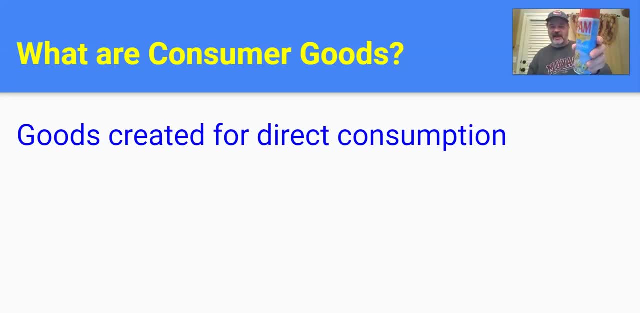 the product placement. here we go: Uh, this is Pam, Uh, Pam is uh for baking. And so what you do is you spray this nonstick pan Pam on your pan And that way, uh, whatever you're cooking. 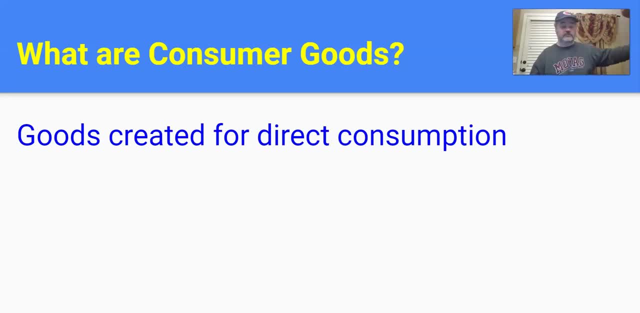 doesn't stick on it. This is a- um uh, consumer good. Um, this right here, uh, in case you're going to have a pizza today, uh, this little pizza cutter right here is a consumer good. Very, very important. 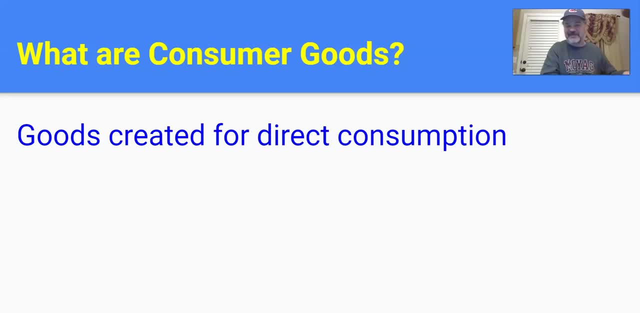 Um, Ooh, I love this. Okay, Jumbo playing cards Isn't that cool. Look how big these things are. These are big, giant playing cards and I have like two sets. Okay, So you could like. you know it's like a fan or whatever. 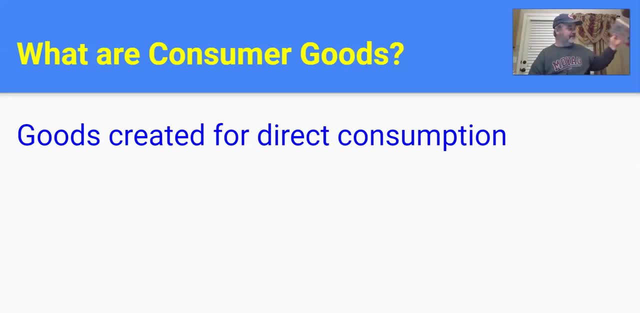 but this is actually a consumer good. It's a novelty, but it's a consumer good. Uh, this is. I have cats. Uh, this is a little, uh, cat toy ball. It's got a little mouse thing in it And the cats like bat this around and sometimes they play hoops. 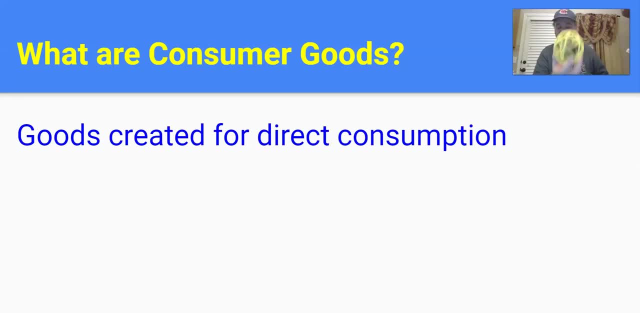 with it. You know, and I've got like: no, I don't anyway, but this little cat toy is a consumer good. Now, the consumer for this is, uh, the cats, but uh, actually it's for my entertainment as. 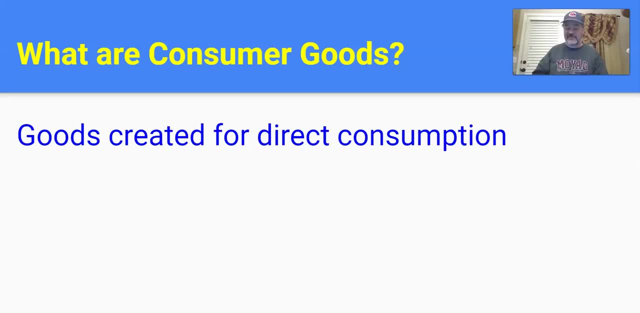 the cats play with that. Um, now, uh, this is really cool. Uh, you know, I I drink a lot of water. This is, uh, uh, this is something called liquid death. Okay, And liquid death is actually. 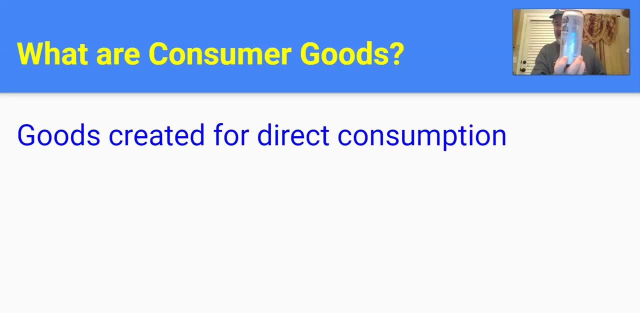 designed to murder your thirst. Okay, And so I'm going to open this can of liquid death. Hmm, Yep, Mountain water. Ooh, it's cold too. So I've got the mountain water. Uh, it's an interesting product. We're going to be talking about liquid death, actually in this class. 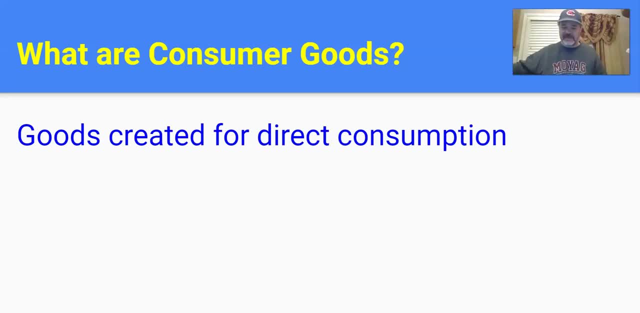 as we move into supply and demand. it's very, very interesting model they have in this company for selling things. And then one more thing I'm going to show you real quick, obviously is a cell phone And uh, this is a very complex uh item, but this also is a consumer good And um and so, uh, as we 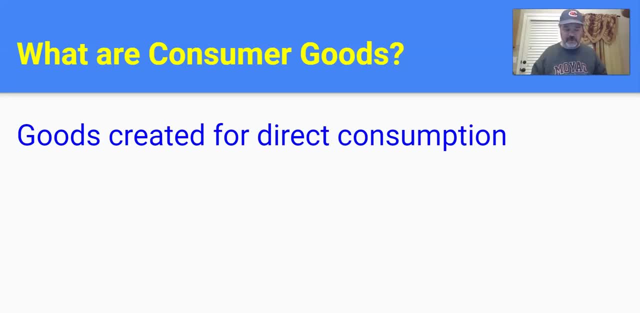 look at this here: um, these are all consumer goods. Now let's move on. Now we have consumer goods, and I've shown you some examples of those. Those are for direct consumption. Now we're going to talk a little bit about capital goods. and a capital good, um, are goods that are created for. 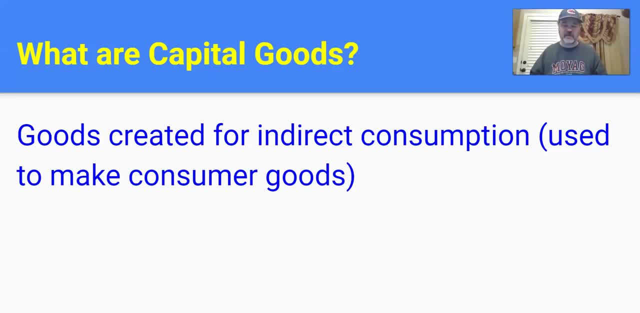 indirect consumption used to make consumer goods. Okay, Now I'm in my home And so I don't really have a lot of um capital goods here, Um, and so when you're talking about this, you're talking about like a factory, you might have a machine, uh, that makes um the cans. 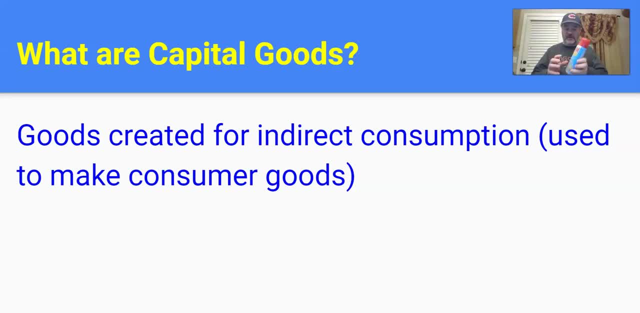 from okay, And so that machine is considered to be a capital good. You might also have a machine that makes the lid, which is a little plastic lid, here, It'll um, uh, that is um, a capital good. 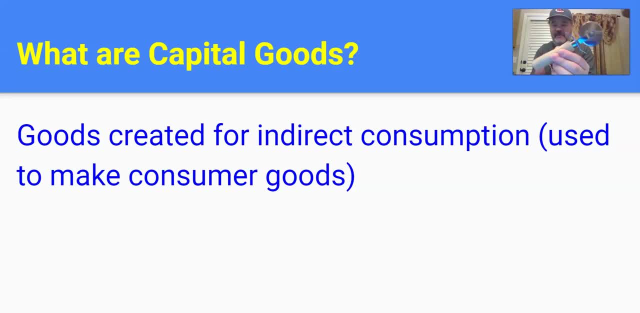 Now I do suppose that if I take this pizza cutter here and let's say I started a little business in my house and I'm making pizzas out of my house and I'm selling them, uh boy, I better have all the government agencies. 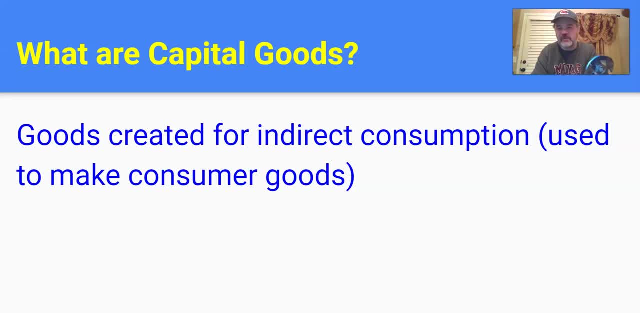 The hot paperwork done on that one. But anyway, if I were to make you know, do this in my own house. this is, uh, this is a consumer good. I mean I'm going to use it for myself, but if I'm 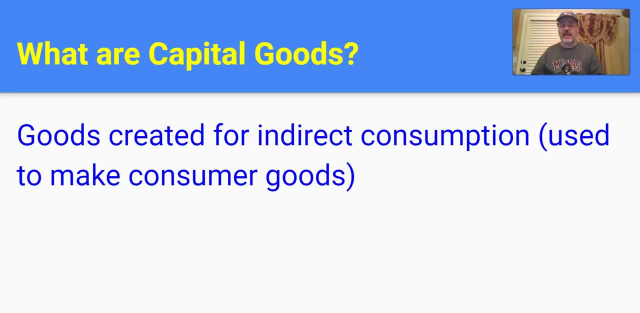 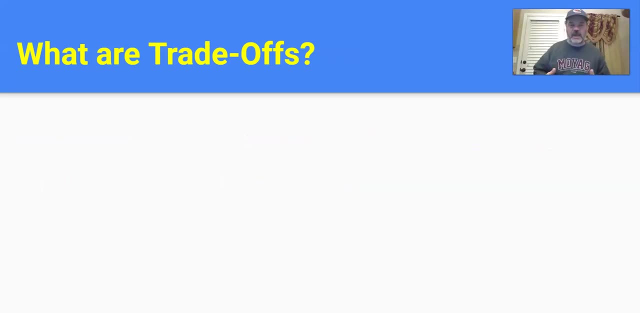 going to have a business here, then this also is considered to be a capital good, And so put that down there. So capital goods are for creating consumer goods, And it's just really simple to understand. Now we're talking about scarcity- Okay, The unlimited wants and limited resources, And we're going to be talking a lot in this class. 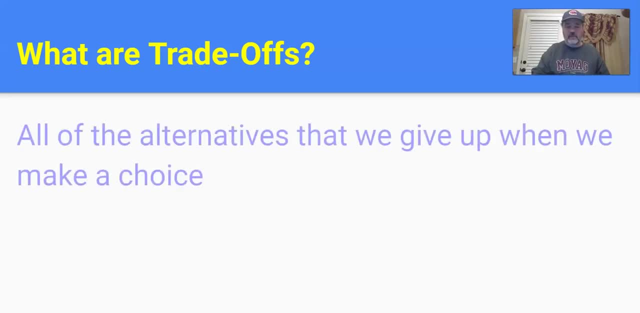 especially in the next unit, about something called trade-offs. And what exactly is a trade-off? All of the alternatives that we give up when we make a choice. Okay, Now, um, let me show you what I'm talking about here. Uh, let's do this as an example, Okay, So here's an example. 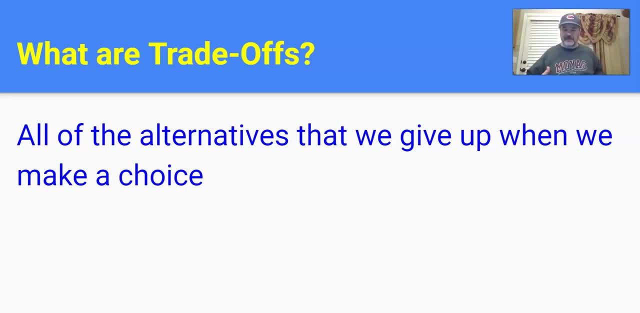 I'm thirsty, Okay, Now, um, I can only imbibe so much fluid in my body to quench my thirst, And so, um I I could, uh, drink some of this milk. Okay, Drink from the jug. Don't do that at home, Moms don't like it. 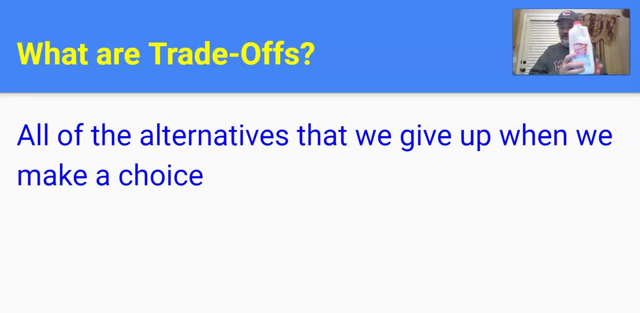 when you drink from the jug. Um, except I don't live with my mom, So that that was. yeah, I could do it, I guess, if I want to. but, um, the trade-off here is: I mean, I could drink milk, Okay, Or I. 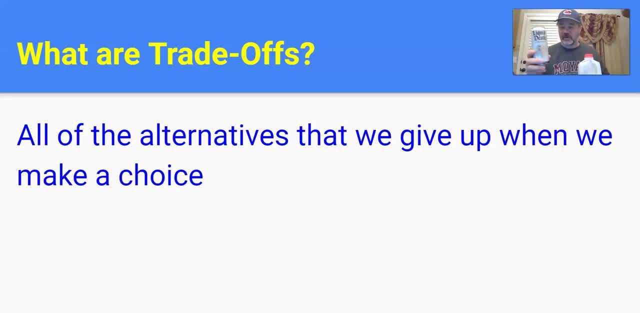 could drink my liquid death. uh, mountain Water, canned water, Okay, And. and so I have to make a choice. What do I want? Okay. So the trade-off is: I've chosen to drink water, Okay, And the trade-off is: I've given up, uh, drinking. 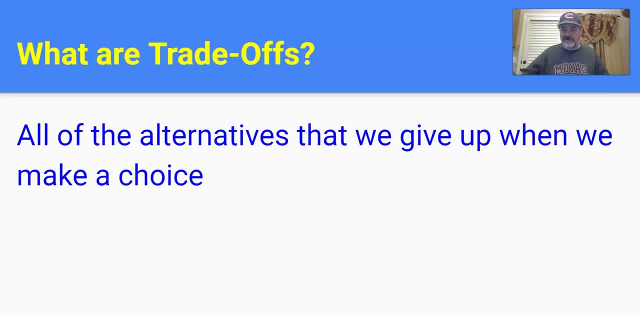 milk in this case. I mean, I guess I could drink both, but you know, but uh, at the same time, but that would water down the milk and it wouldn't taste very good. So I'm making a trade-off. 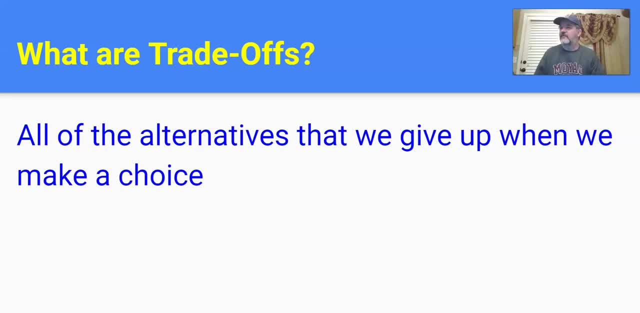 Now other trade-offs, uh deal with other things, like, for example: uh, it's uh like when I'm making this video right now, it's about 15 below zero outside, So I am going to stay inside today. Why? Because I don't want to go outside. So, uh, I have chosen. 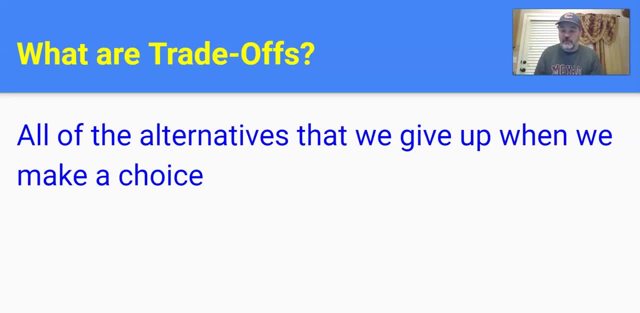 I've made a choice to stay here at home, um, as opposed to going outside and getting frostbite. That was the trade-off, And I think it's a pretty good trade-off, uh, to stay in my house, And so we're. that's a weird example, but this is what we're going to be talking about in here. 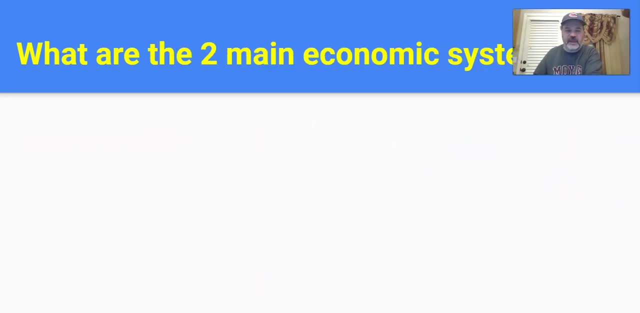 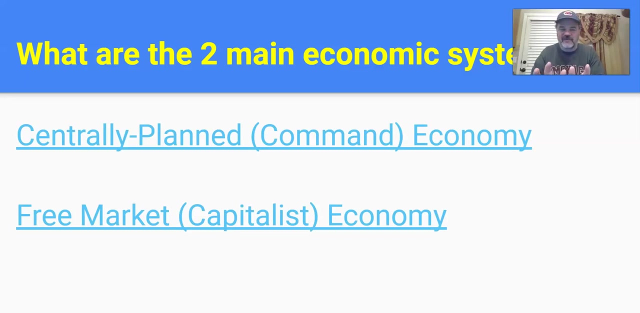 With trade-offs. Okay, Let's take a look at, um, the two main economic systems that we're going to be talking about in here. Um, the two main systems that we're going to be dealing with in this class are what's called centrally planned or command economies. Uh, sometimes you think of it. 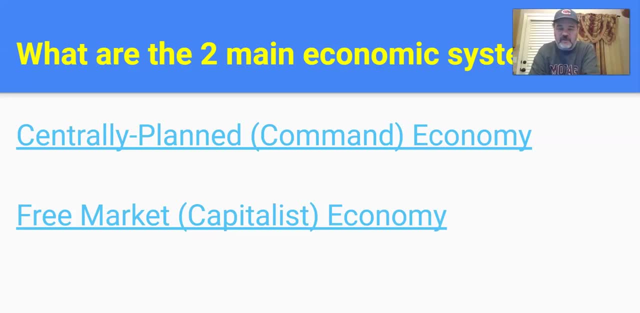 as communist. Okay, And that's fine. And, by the way, on this screen you will see that there is a link. I will include the link to this Very strange video, Um, in the link below. you don't have to watch the whole thing, but if you 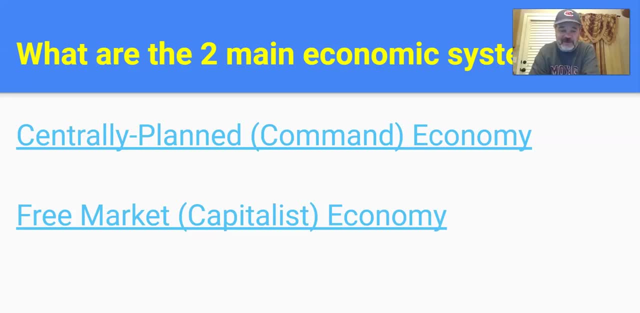 watch a little bit of this video. it's it's quite humorous, Uh, it's kind of scary too, Um, and it kind of shows you, uh, during the cold war, about what a command economy was. And then the other type of economic system that we're going to be talking about is called the. 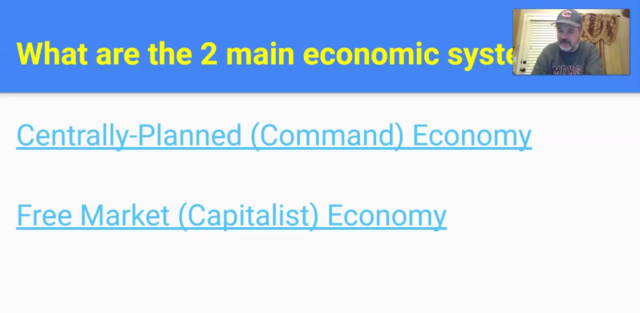 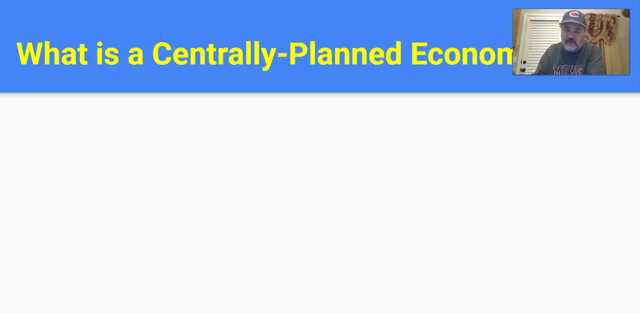 free market or capitalist economy, And that's kind of the one that we live in today And we're going to be talking about that, what that is. Now I guess you could say that, uh, you know that, well, we'll get to that in a minute. What is a centrally planned economy? Um, and we're 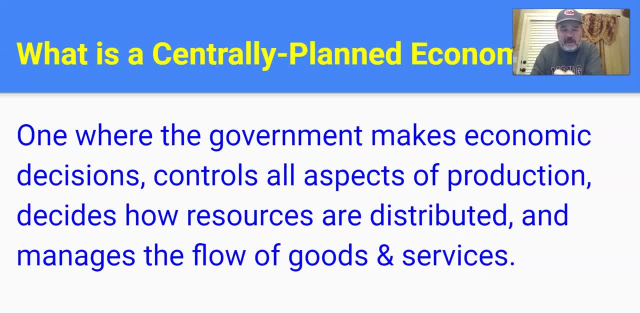 going to get to this third one here in just a moment, but let's start with this one. A centrally planned economy is one where the government makes economic decisions, It controls all aspects of production, It decides how resources are distributed and it manages the flow of goods and 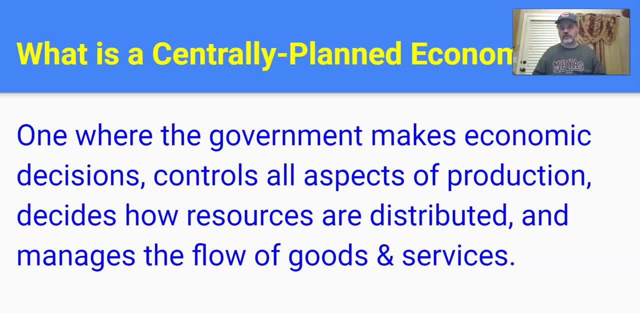 services. In other words, you know communism. okay, The government will swoop in. It owns everything, It does everything, It decides how the resources are divvied out and distributed. It manages everything. All aspects of economy are controlled by the government, a centrally planned. 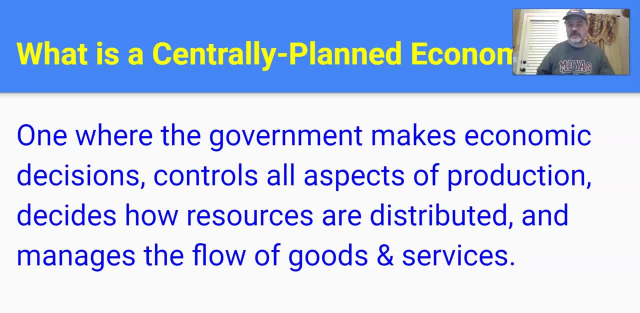 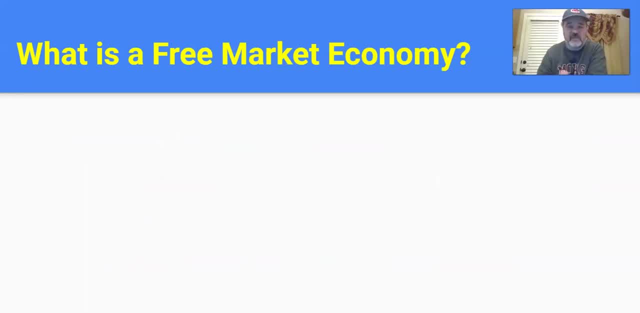 economy, or the other word for it, is a command economy, because the government is commanding how that is going to be run, as opposed to what you think of as the free market economy. and the free market economy- And a lot of you think that the United States is this- this is one where the 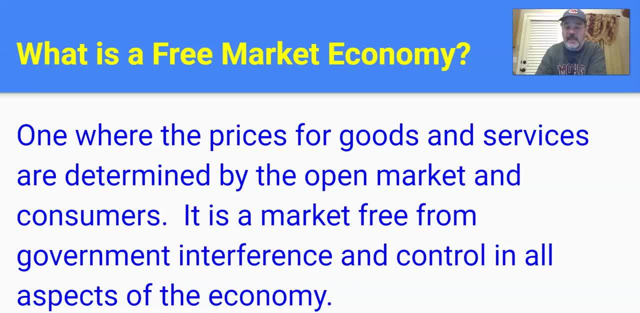 prices of goods and services are determined by the government, And the government is commanding what is determined by the open market and consumers. It is a market free from government interference and control in all aspects of the economy. So you know when I walk out my door. 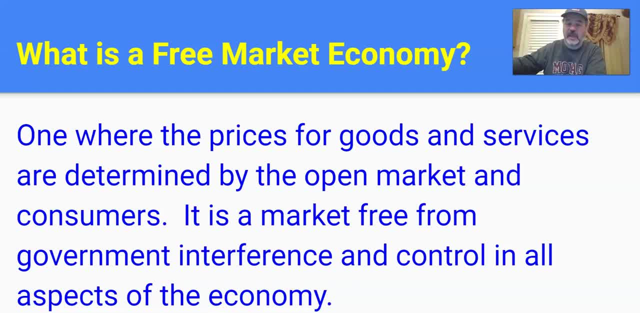 and I want to go buy a liquid death. okay, Uh, if I want to go out there and do that, well, I got to go find the person that's selling it. They're going to set the price. I'm either going. 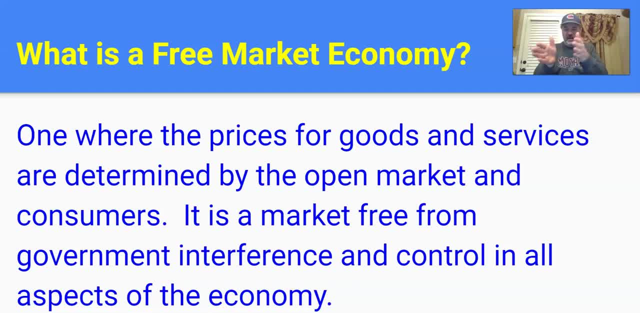 to say no, I don't want to buy it at that price. We might dicker a little bit and get that down to the brim, where it's price that he agrees to sell it to me for, and I agree to buy it, And so you. 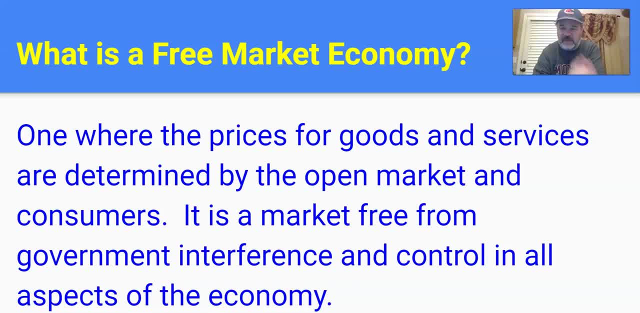 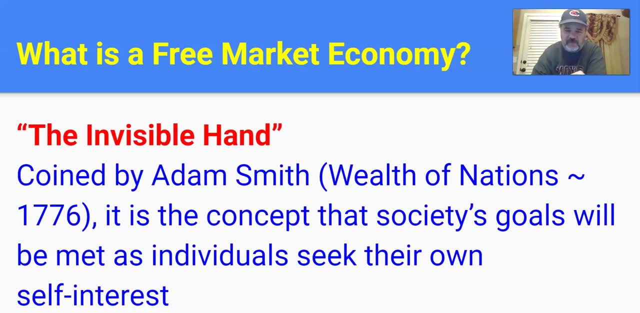 have this free market economy and the government is not involved in that whatsoever. Okay, Not at all. Do we have that in the United States? No, we do not. And so what do we have in the United States? I'm going to get to that in just a moment. I want you to be familiar with this, Adam Smith. 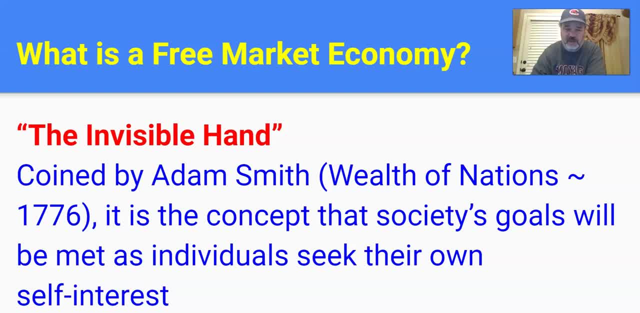 uh, Adam Smith, that was a squat and he was from Scotland. He wrote a book called the wealth of nations And coincidentally, he wrote it in 1776.. Didn't have anything, anything to do with our revolution, Uh, but he wrote this book and in it, um he. 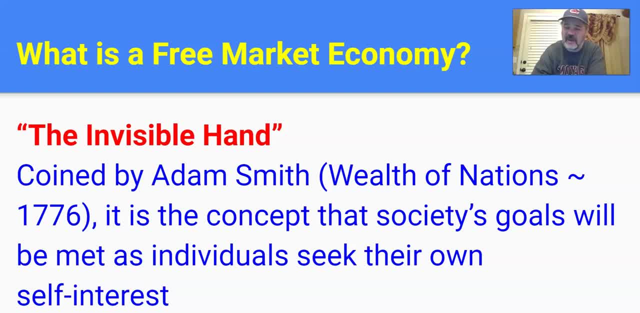 talked about something that was called the invisible hand. It is the concept that society's goals will be met as individuals seek their own self-interest. Wow, That seems to be a mouthful. It is a philosophy on human behavior and that human behavior and interaction. 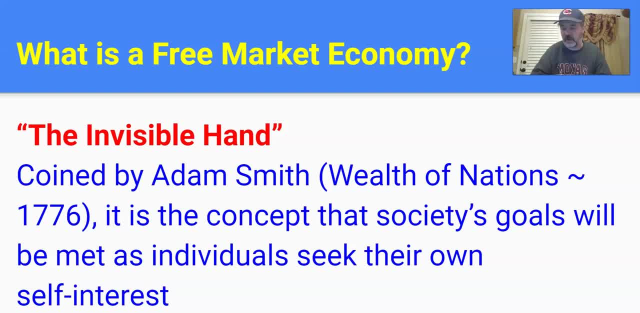 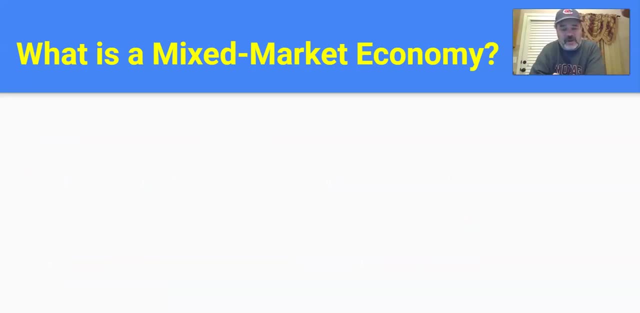 between human beings through an invisible hand is what he called it. We'll decide the free market and we'll decide prices of goods and services. We're going to be talking a lot about this as we move into the- uh, deeper into the course. Now, is the United States a free market economy? 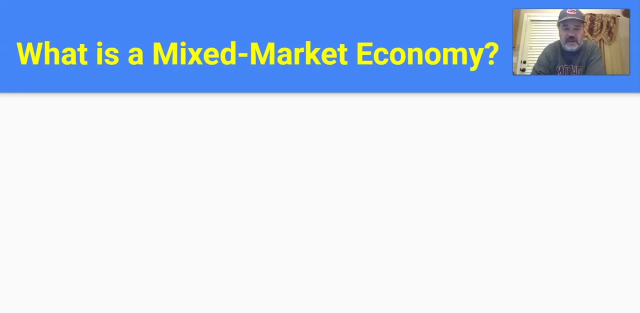 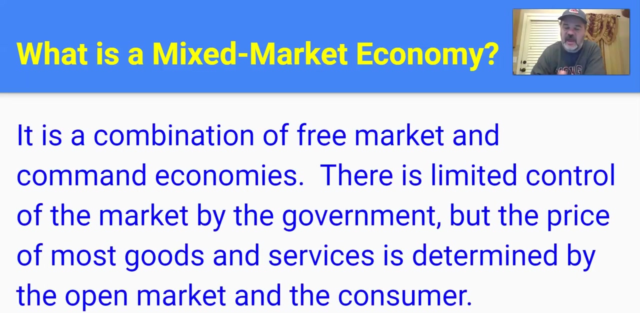 Probably not, because the government is involved in our economic affairs to some degree, but not to the degree of like the Soviet union or China. Okay, You have what is called a mixed market economy. This is kind of what the United States is. It is. 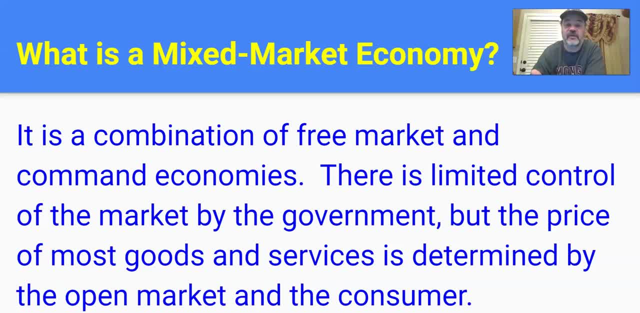 a combination of free market and command economies. There is limited control of the market by the government, but the price of most goods and services are determined by the open market and the consumer. Okay, So there is this uh market system that will affect prices. 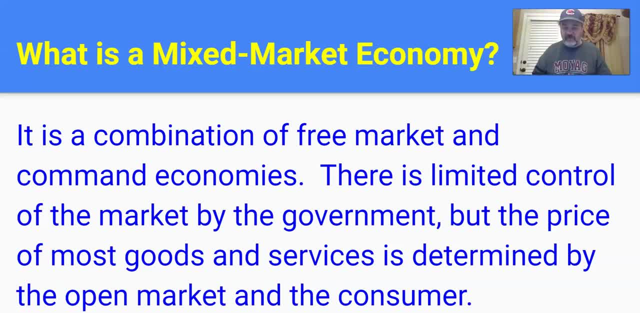 uh supply and demand and all of that. However, the government is involved in some degree in a limited amount of uh market economy. So, uh, the government is involved in some degree in a uh degree. uh, for example, you know, like like liquid death When we come back to liquid. 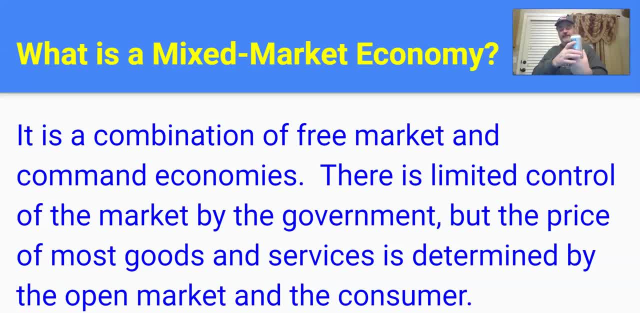 death again. um, on this, can there has to be um, uh something on here about what's in here And it says there's just water as mountain water. Okay, Um, this milk that I had a few minutes ago. uh, on the back, the government requires that there are um uh nutritional. 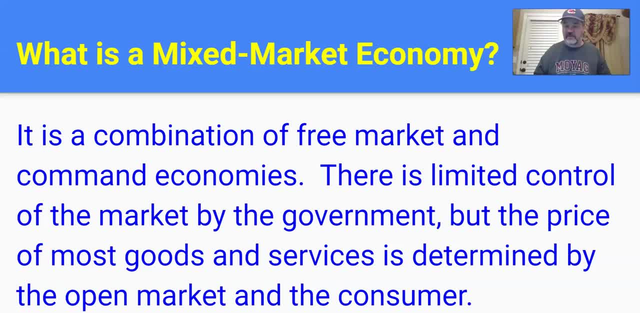 facts on here That's controlled by the government. Uh, sometimes the government will control slightly amount of milk that is produced, using various ways and means to do that which you've learned about in American history when we were in the Great Depression, Or you could talk about the 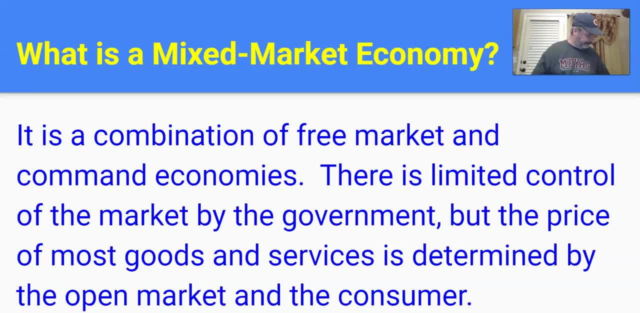 safety of some items. okay, For example, you know these giant playing cards. okay, They're made out of plastic, but is the plastic a carcinogen? So the government will decide what kind of plastics can be used to make this particular item. okay, So the government is involved in a mixed market. 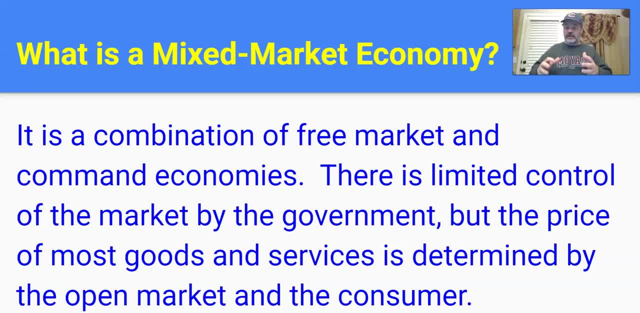 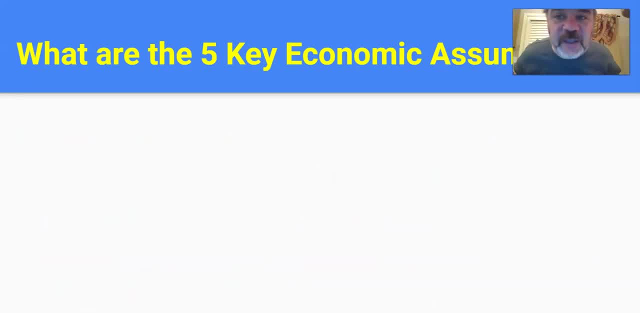 economy to some degree, but not totally like a command economy. Now, this is really really, really, really, really important, really important, okay- that you need to know, And they are called the five key economic assumptions. You need to know these, You need to know them, You need to. 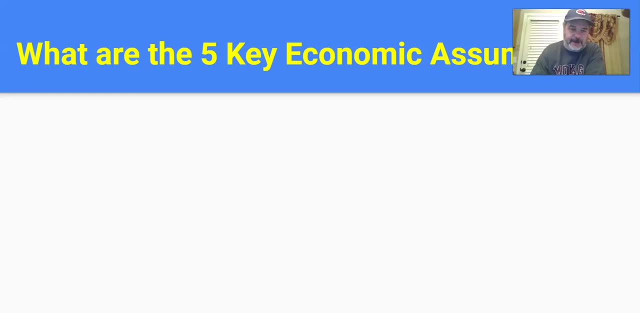 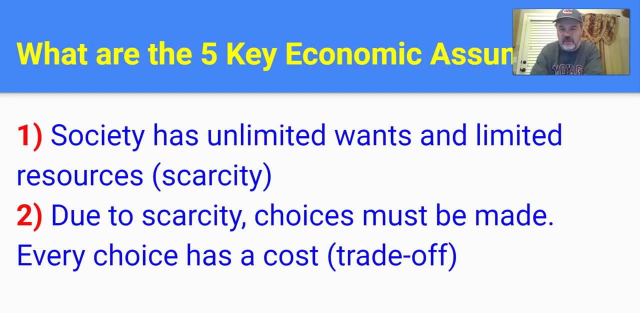 know them. I don't know how much of a big hint I can give you on this. Number one, and this is an assumption that you have have to have as we move forward in this class, as we learn about economics, society, and we've already 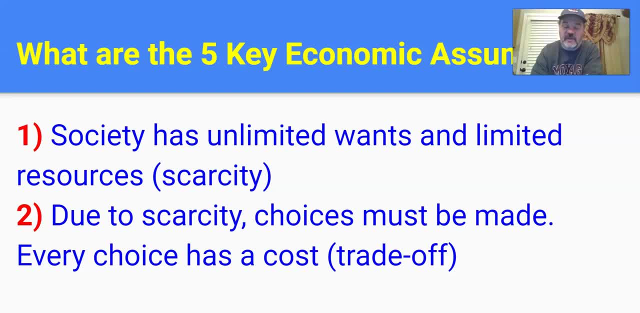 said it. okay, society has unlimited wants and yet it has limited resources. so in economics we must assume that there is scarcity. some things are more scarce than others. i mean gold, for example. that's really, really scarce resource out there. okay, uh. water, on the other hand, uh, not as scarce. 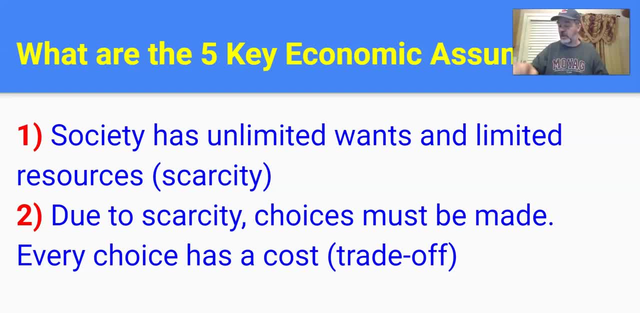 but clean water, uh yeah, it is scarce. mountain water might even be a little more scarce, but society has unlimited wants and limited resources. first key economic assumption. number two: due to this scarcity, choices must be made and every choice has a cost and that's called a trade-off. okay, so the first two key economic assumptions. number one: there is. 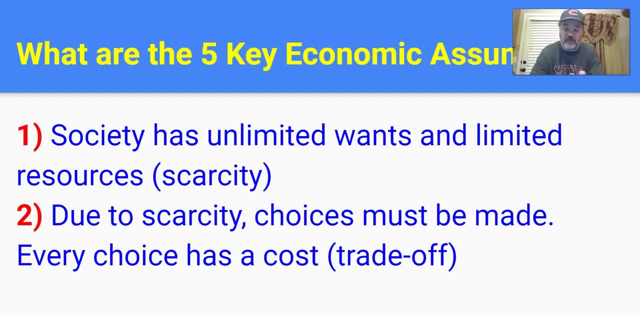 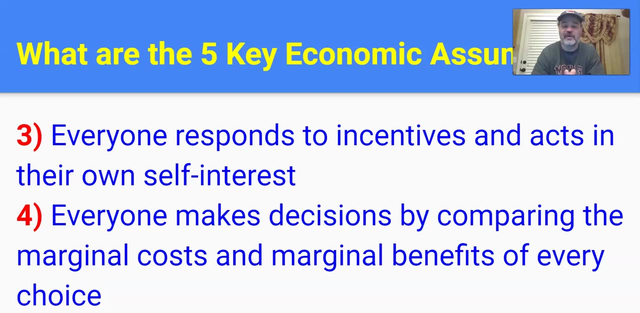 scarcity in the world and number two, human beings. people, uh, society has to make trade-offs because of those choices due to scarcity. the third key economic assumption is that everyone responds to incentives and acts in their own self-interest. okay, in other words, you're not going to be able to make a profit out of it. you're not going to be able to make a profit. 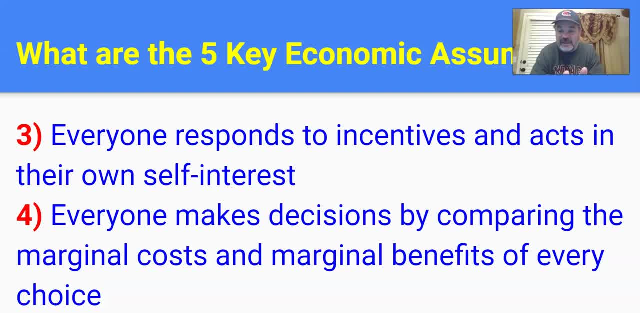 out of it. you're not going to be able to make a profit out of it. you're not going to make a profit. greed, we are greedy little people. uh, greed is good, uh, as gecko said in the 1980s movie wall street: okay, so everybody responds to incentives and they act in their own self-interest. 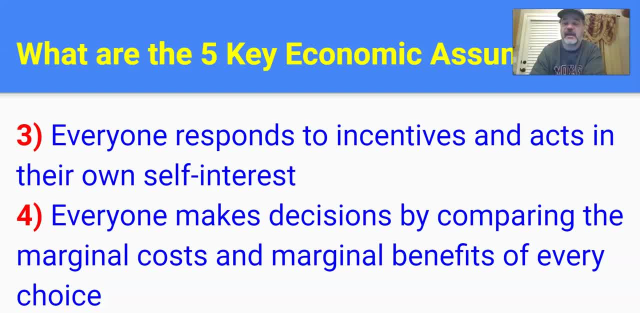 okay, so we're looking out for ourselves. however, in an economic system, in a free market or mixed market system, that greed can be used as a productive means of making goods and services for everybody and actually increasing the production of those goods and services. so, number three: everybody responds to incentives and acts in their own self-interest. number four: 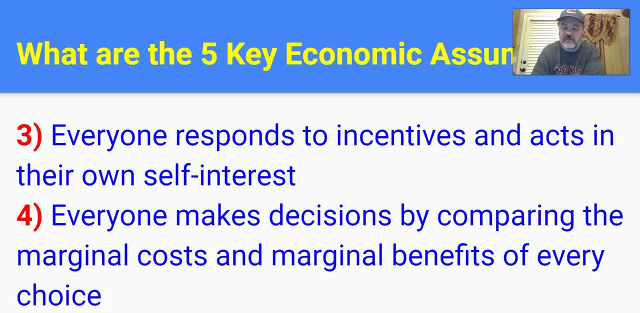 of these five key economic assumptions. everyone makes decisions by comparing the marginal costs and the marginal benefits of every choice. now, what does that mean? okay, here's what it means. whenever you see the word marginal, okay, i want you to think of change. okay, it means change. so 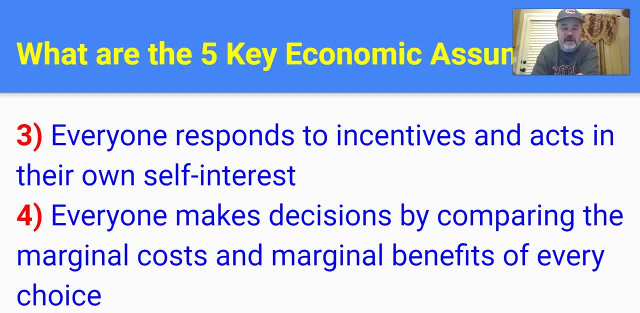 let's reread. let's reread this: everyone makes decisions by comparing the change of costs and the change of benefits of every choice. okay, so when we look at marginal cost, we look uh at the cost of production in in the change uh of the total cost. okay, for example, um, you know, if, if i'm going to make, let's say i'm 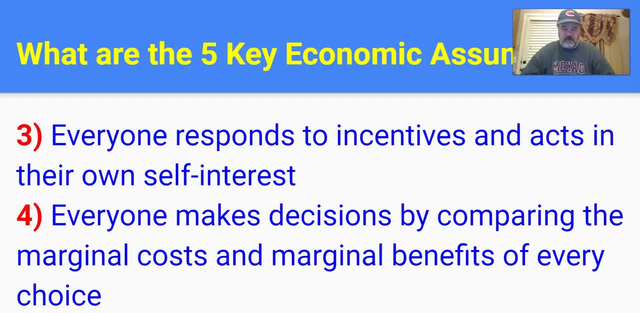 a business owner and i'm, i've decided to make donuts, okay, uh, you've got to look at the marginal costs of the equipment that i'm going to buy and compare that to the marginal benefits of how well the production is going to be okay, and so we have to take those things into account. 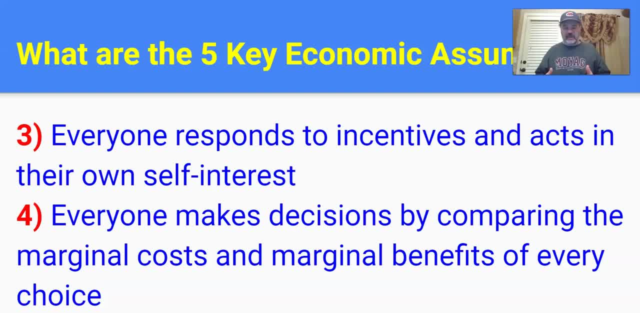 as we create the donuts, okay, or anything, or something that you do in life, okay, some things that you do have a cost, but that cost has a benefit. for example, you know, i could choose just to drink uh milk all day and at my age, if that's all i drank, i'd get fat pretty quick. 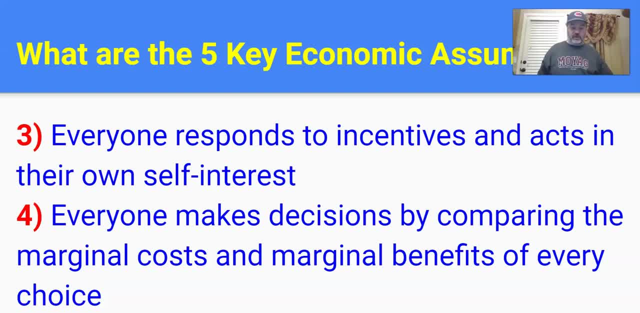 okay, so i like milk, um, i, you know i'm going to go out and spend, you know whatever. it is three, four dollars for this milk, uh, but you know, and the benefit is, you know, it's going to make me, it's going to make me feel good, i like milk. okay, uh, but there is a cost to that and that is. 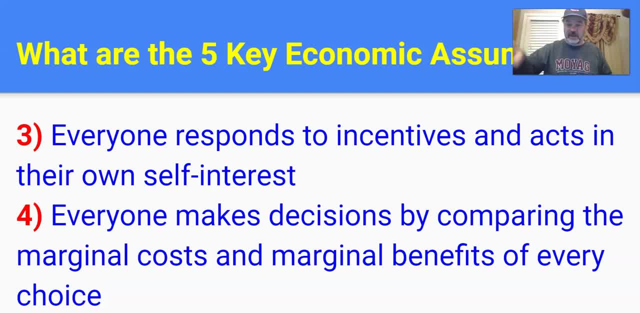 my width okay, or i could drink water- okay and i like this water. uh, there is a cost to that. okay, it costs me money and there is a benefit to it: it quenches my thirst, um, and it doesn't make me. so you have to look at the changing cost and the change in benefits. very, very important economic. 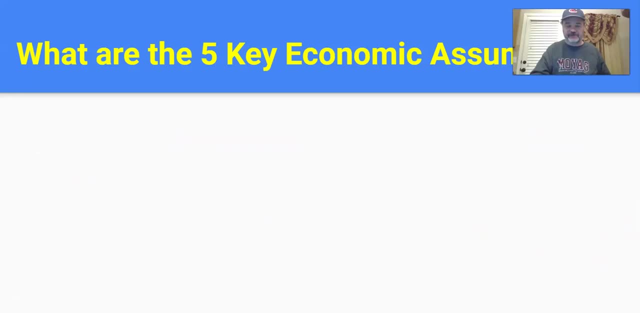 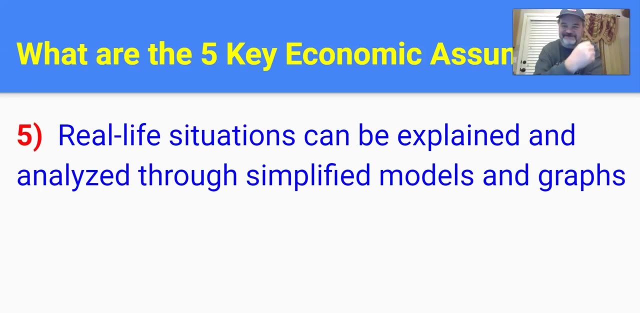 assumption. okay, the last one here is very, very important: real life situation and- and, by the way, this is you really have to go with this- you really really have to go with this assumption- real life situations can be explained and analyzed through simplified models and graphs. okay, now 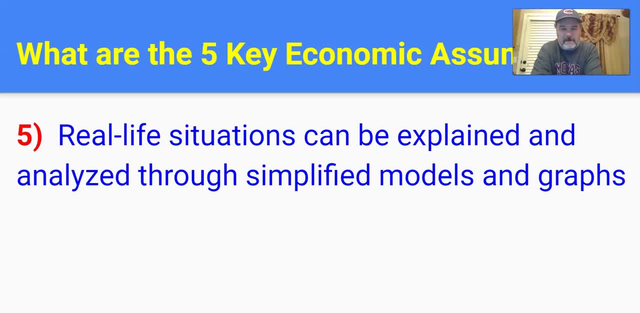 some people say that's a stretch. okay, how do you measure human behavior? that's pretty tough, and so if you're going to be an economist, if you're going to study economics, you have to believe that you can analyze through simplified models and graphs. you can, you can. 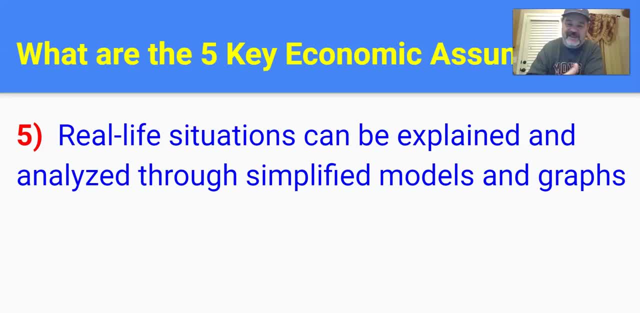 actually model out real life situations and predict behavior of consumers, and some people say that's not possible. um, but if you're going to be an economist, if you're going to study economics, you have to assume that this is possible. it may not be very accurate, but this is a science. and this last assumption: 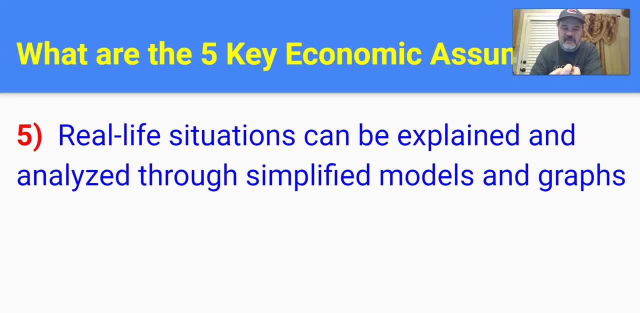 is what makes economics a science. it's the analysis through simplified models and graphs, just like you would do when you're studying bacteria or you're looking at plant growth, or if you're looking at, um, i don't know, radiation effects on rocks from the sun, i don't know. yeah, i can make up all kinds of things that. 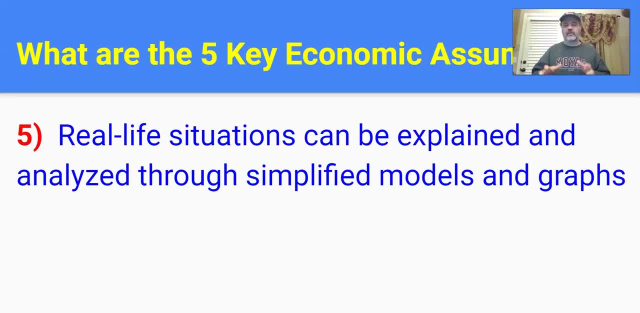 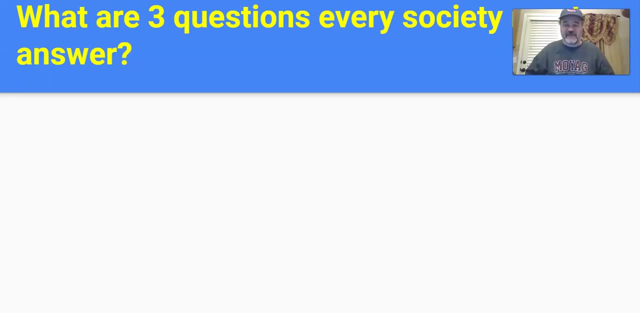 scientists do, but this kind of scientist is measuring human behavior with regard to trade-offs and scarcity and all of the other things which we have just aforementioned. okay, now, this is the last thing that we're going to talk about here. what are the three questions? every society must? 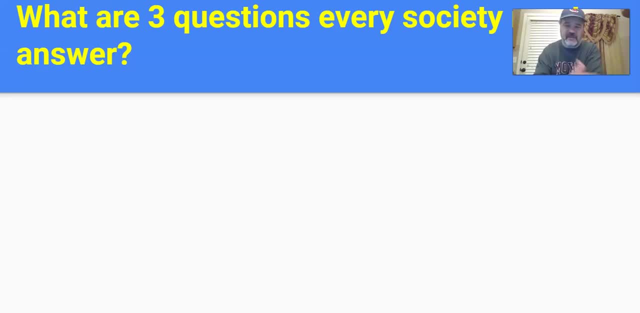 answer. um, and this is, this is kind of a something that is not like every economics class you're going to have these questions in, uh, but this is something that i thought was a very good, thought-provoking thing to kind of end this small unit on what are. 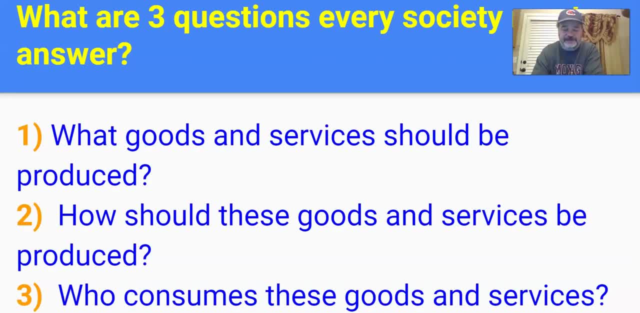 the three questions every society must answer number one: what goods and services must be produced. i mean, we have to decide as a society what we're going to produce. okay, um, you know, for example, are we going to make the old analog telephones okay, or are we going to make cell phones okay. we're going to have to decide how that's going to happen. 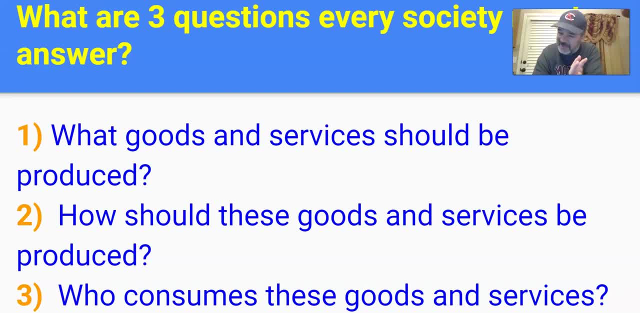 or what we're going to do, what goods and services should be produced at a given time in history. okay, should we be producing horseshoes in mass? i don't think so. okay, not today. now, if you ask me in you know 1868. yeah, we should be making a lot of horseshoes. not so much today. um, number two. 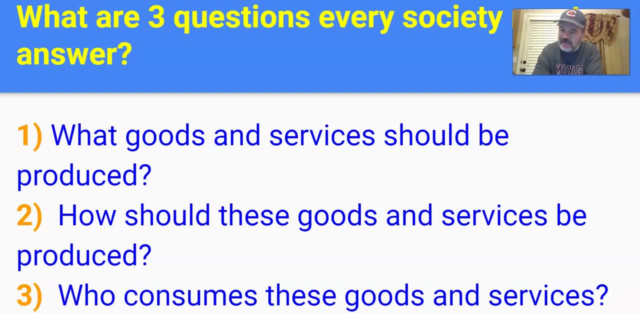 how should these goods and services be produced? okay, that's very, very, very important. okay, um, with technology and all the things that we have today, there are different ways that we can produce those items effectively with a minimal amount of cost, with a maximum amount of benefit. there's your marginal cost and your marginal benefit, based on 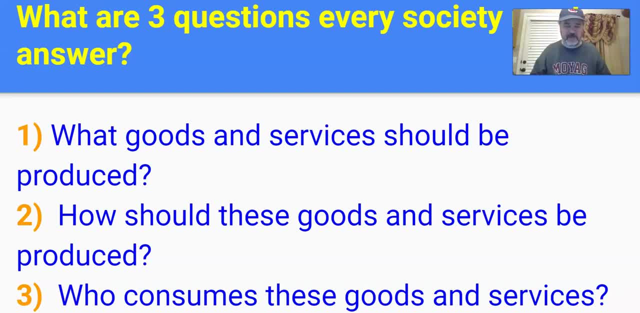 a lot of technological advances, or how many people we should hire, and what type of people we should hire. skilled labor, just manual labor, whatever? finally, who consumes these goods and services? okay, so if you're going to make a cell phone, okay, um, who's going to consume this? okay? how many people out there are going to do that? well, a lot of people. 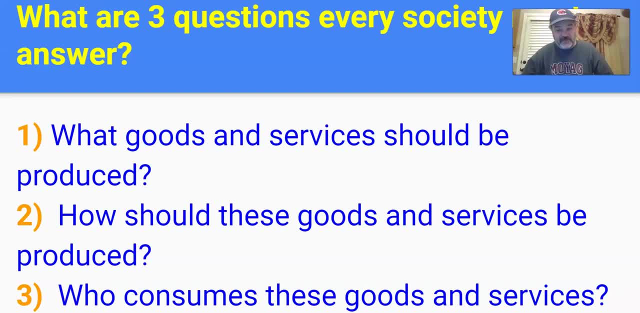 are. you know, i remember in the in the 80s. you know, we had cell phones in the 80s, believe it or not. uh, they were these giant box things. i mean, i could take this little packet here. they were actually bigger than this, these huge boxes. and uh, they, oh, it was a mess, um, and nobody could afford. 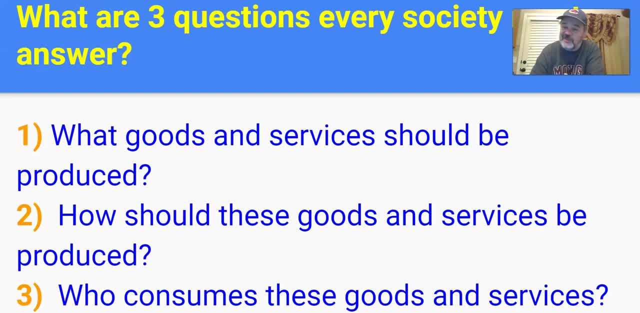 it, there were thousands and thousands and thousands of dollars. okay, so only the rich people could afford those. today, with the way we produce- and this is number two- how should we, these goods and services be produced? today, these can be affordable by anybody. look at, uh, look at uh. elon musk with